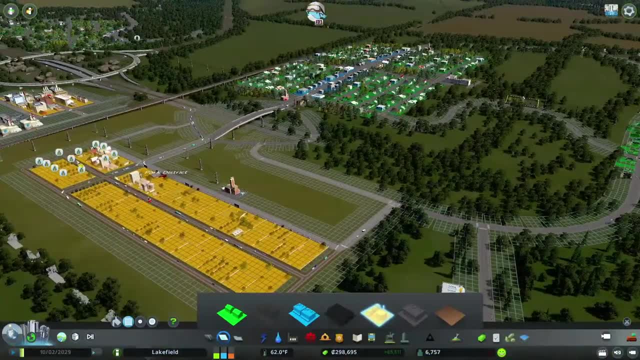 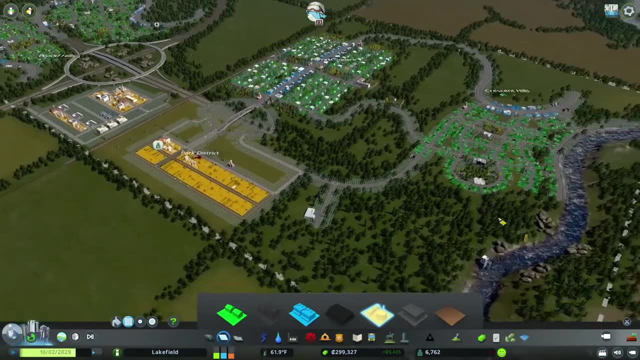 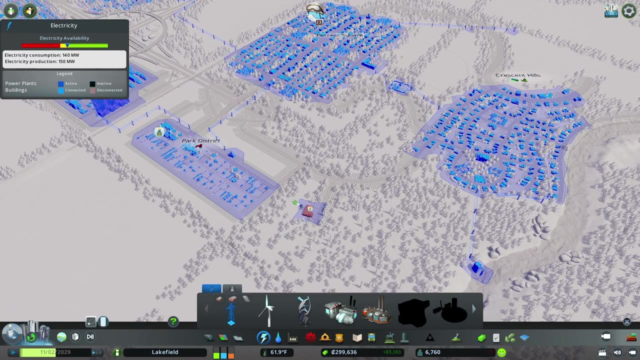 pop him right there. As you can see, it's saying: it's not enough workers Probably having trouble getting from this area over to this area. So that's what the buses are going to do. They're going to help them get around. So let's get some electric to him. There we go All right. so let's go ahead and get some buses run. 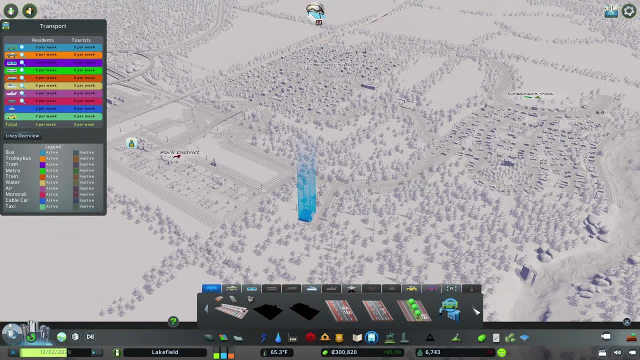 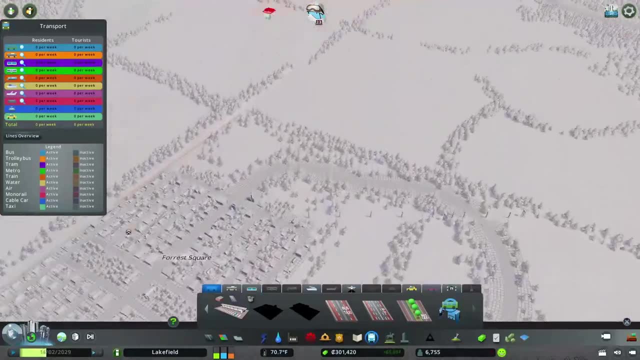 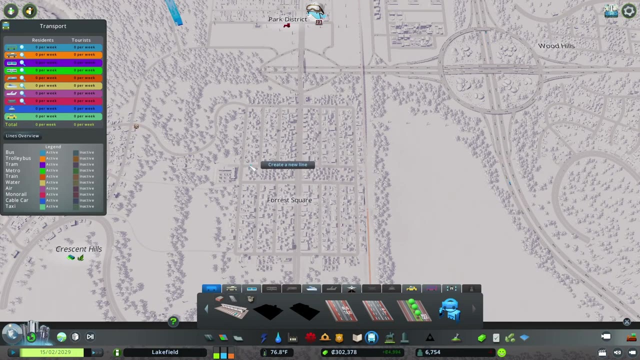 So now we have bus stations or we can just run routes. So we're just going to run routes for now. We don't have any big city right now where we want to add a big bus station, So let's come down into this first area and just make a loop, going counter clockwise, and 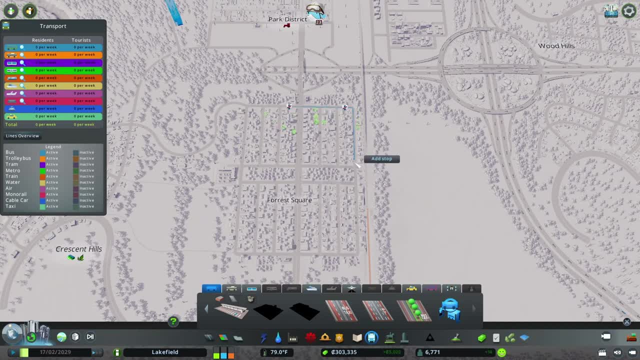 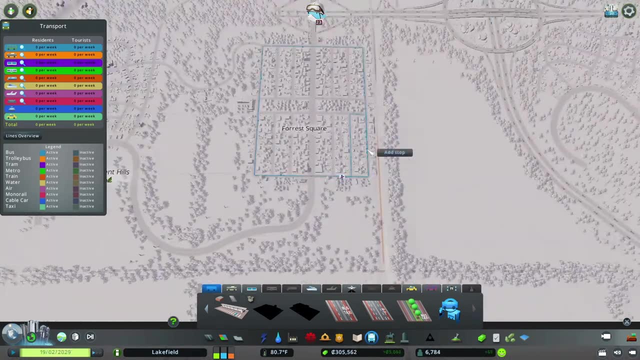 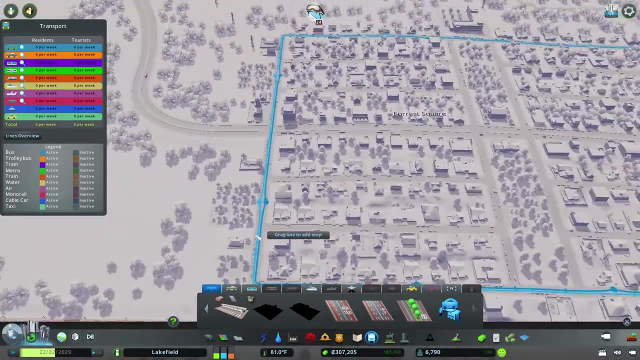 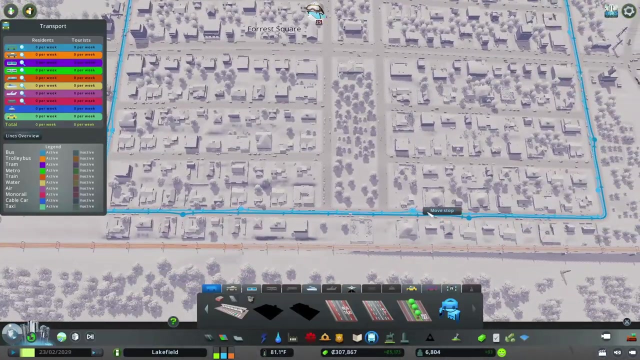 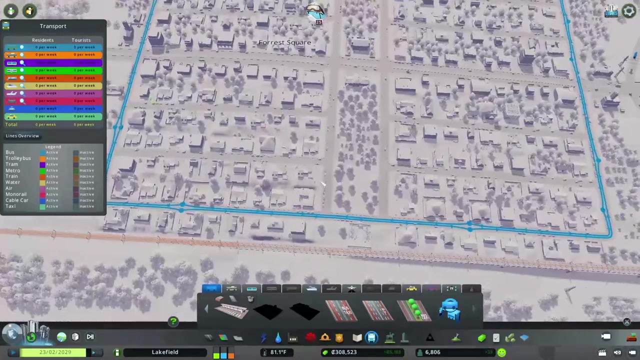 clockwise, Alright. so, as you can see, we have the bus routes and I'm just going to make sure that they kind of line up with each other So you could take this line and drag it down to there, You can grab this line and drag it to there, so they're all kind of even. 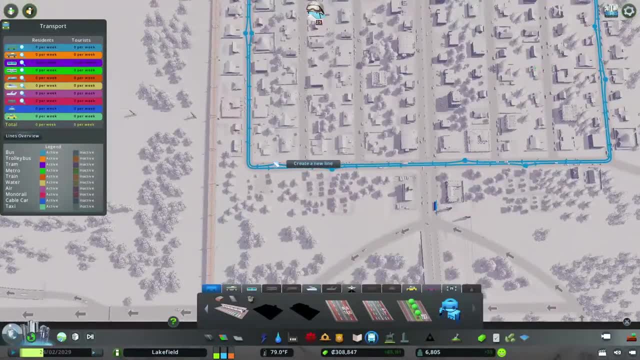 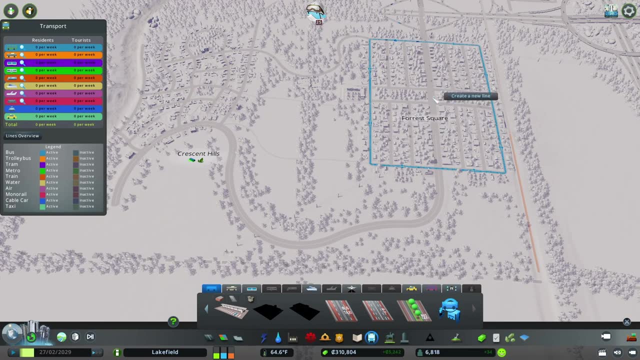 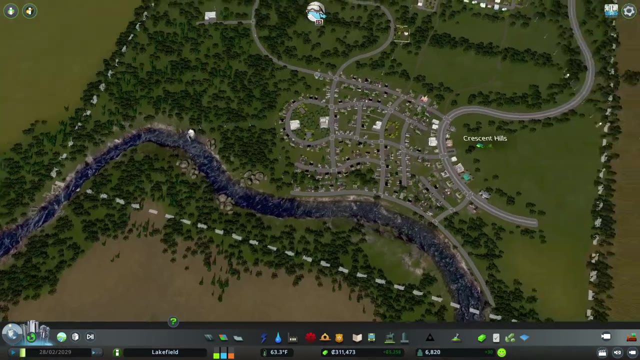 We're going to come on this side and do the same thing. So now you can see their land value is raising because they have public transportation and that makes them super happy. Let's take a look at this other neighborhood Now. we don't have a lot of through roads. 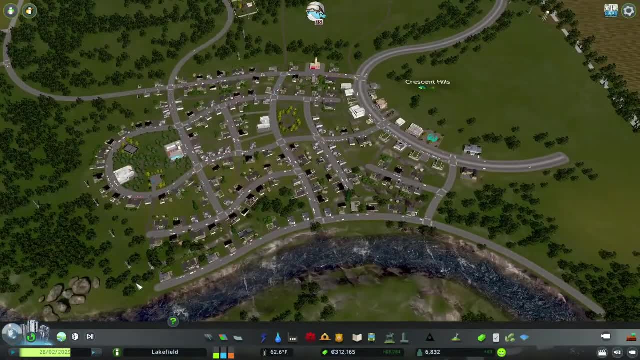 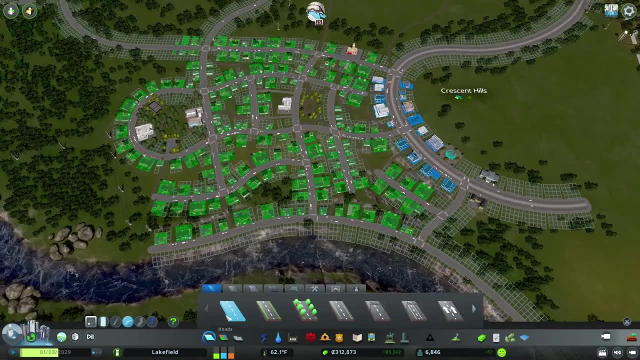 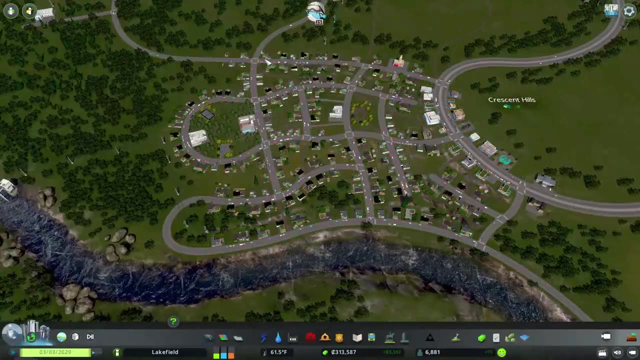 This one does not connect down to this road, so we may connect this one to here and bring this around in a circle this way. So let's take a look. Alright, so now that we connected this road, we can definitely make a nice loop coming around this way and going back. 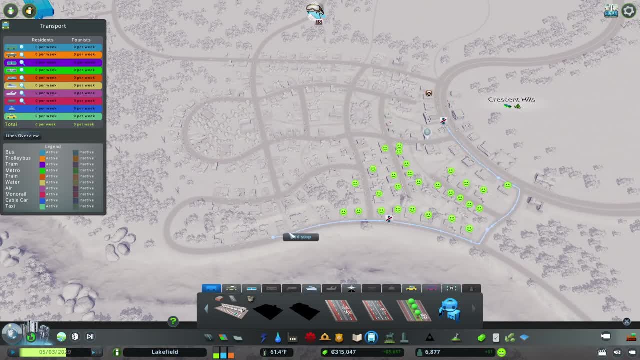 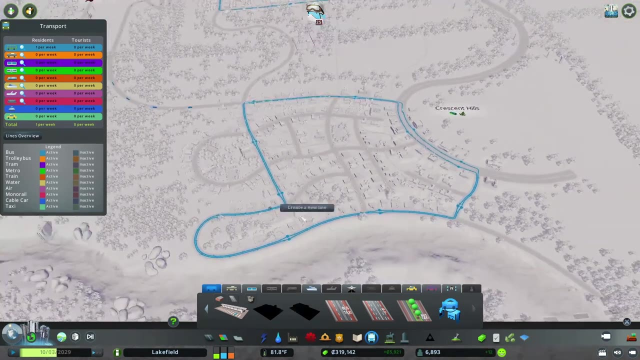 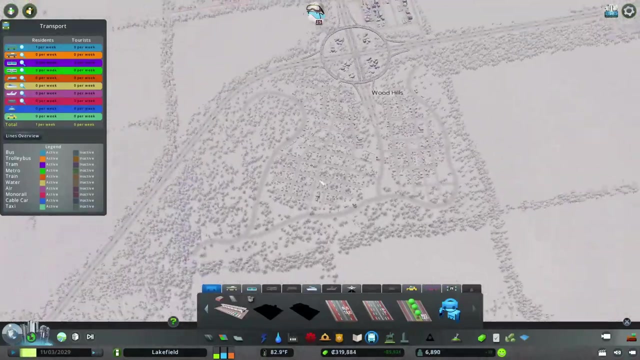 So let's do that. And there we go. Now, eventually I'm going to recolor or repaint these lines so we can tell them apart, But for now let's just keep moving over to here. So let's take a look at this neighborhood. 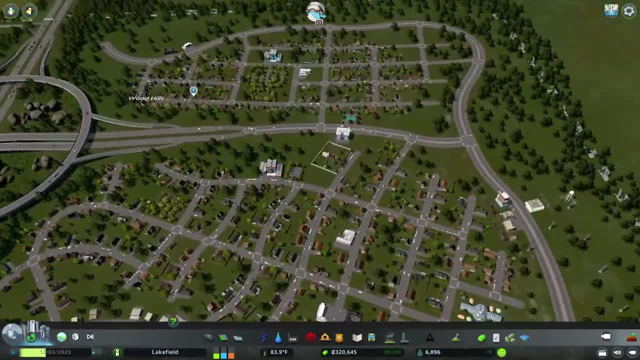 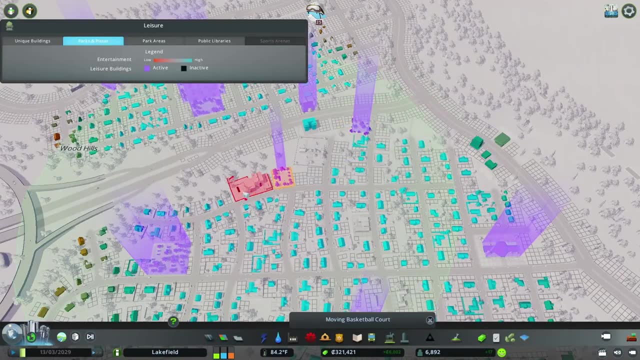 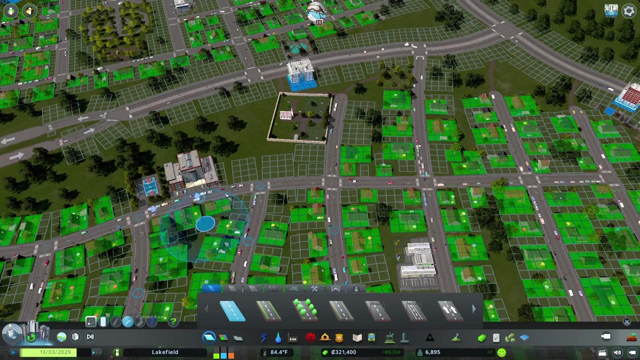 We do not have a lot of cross streets going on in here. What I'm thinking is we may connect this road in here. What is this? A basketball court. We're going to relocate over to there. I'm going to take this road and try to squeeze it in behind the cemetery. 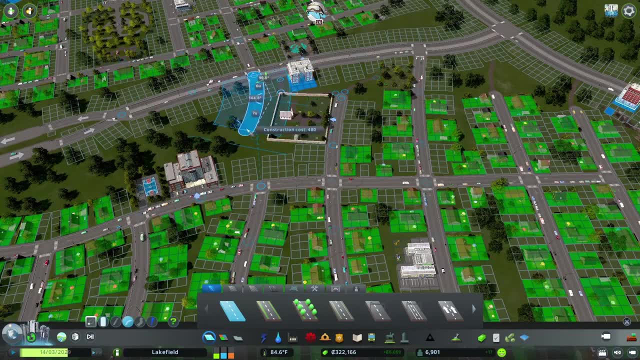 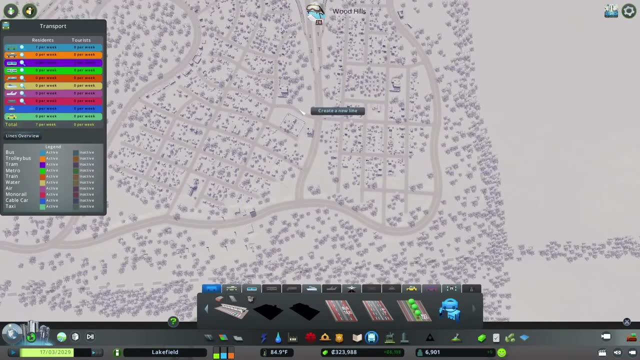 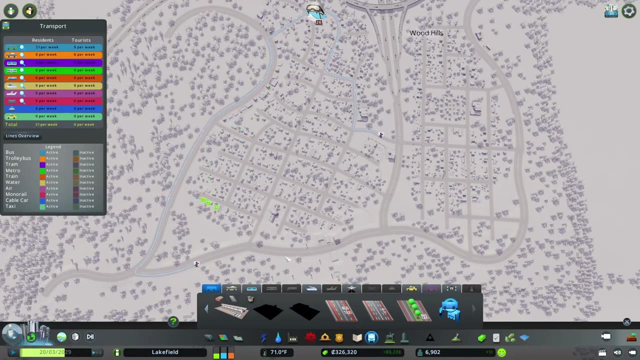 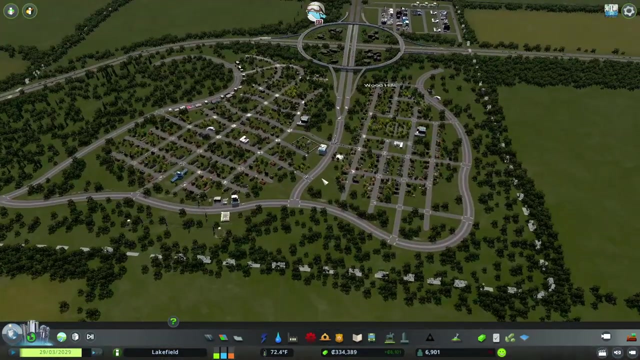 Let's come from this direction. I think that might be a little easier and do something like that. Alright, so now we're set to run our next bus route. Okay, Okay, all right, now that we created three different brush roots for each of the different neighborhoods. 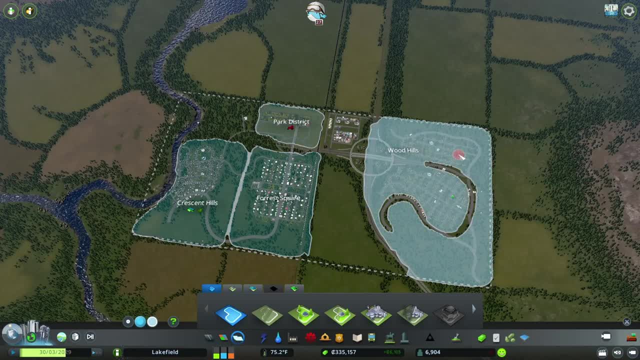 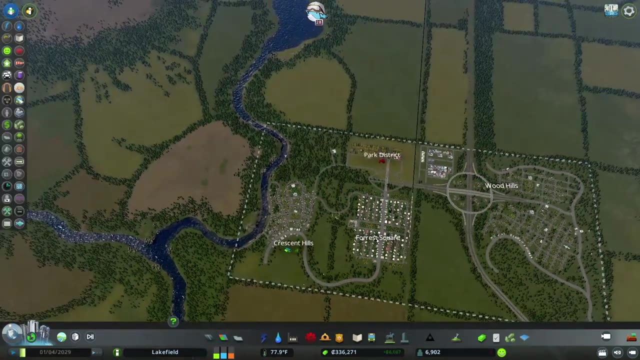 this is Woods Hill. let's just make sure our districts are good. now in here I have European suburbia and I had to take some of the zoning off. it would not fill in for the commercial, so that's okay. no big deal. let's go into our public transportation and get a lines overview. so now, 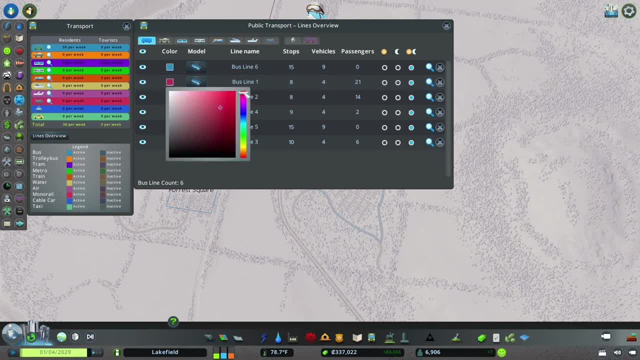 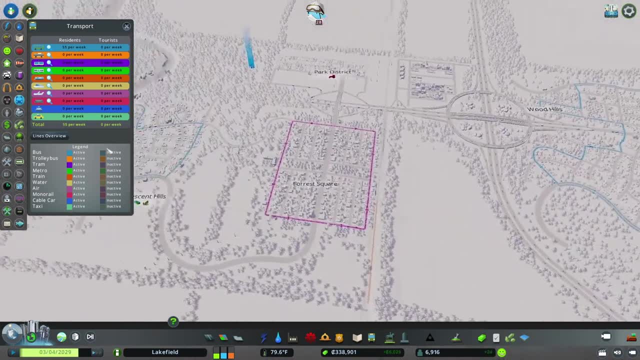 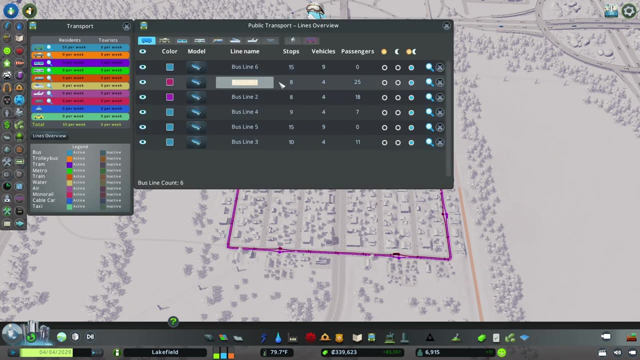 let's take a look here. we're gonna recolor some of these lines. so now line one and two: I just colored pink and purple and we're gonna name that for a square a and for a square B. next we're gonna recolor three and four. so let's keep it as a green. 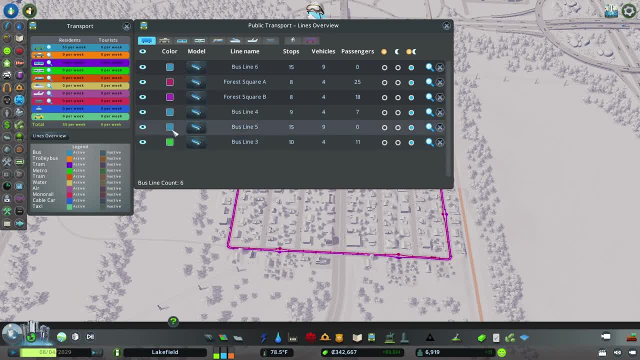 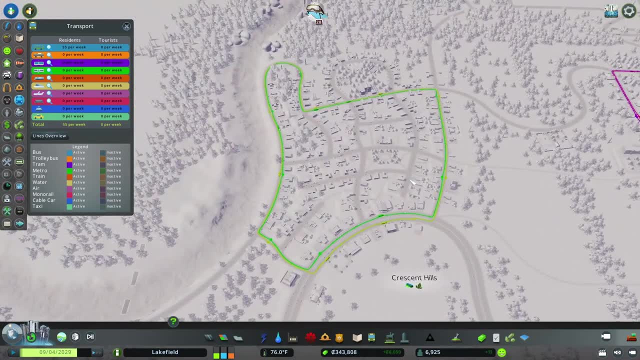 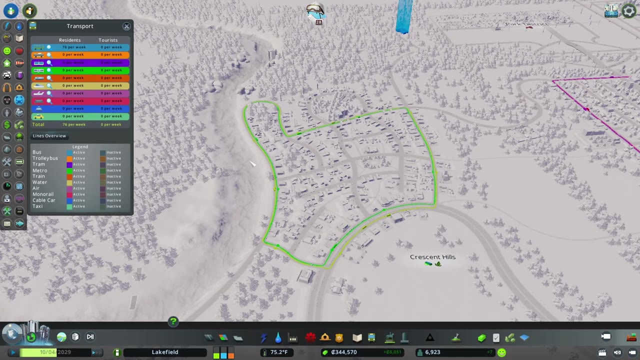 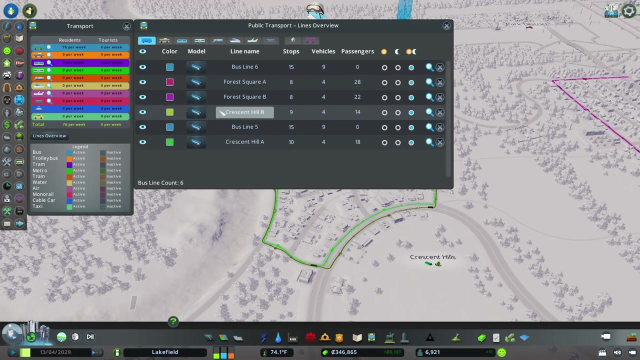 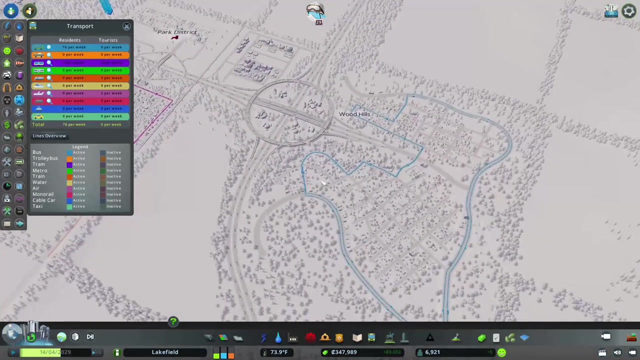 and four will make yellow. so now those colors line up with Crescent Hills. so we're gonna rename the lines Crescent Hill a and Crescent Hill B. all right, so we renamed the Forest Hills, we've renamed the Crescent Hills and now we have to do the Woods Hills. so let's go ahead. we'll do the same thing with these guys. 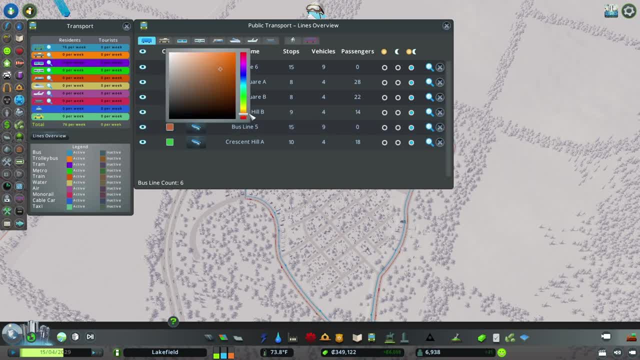 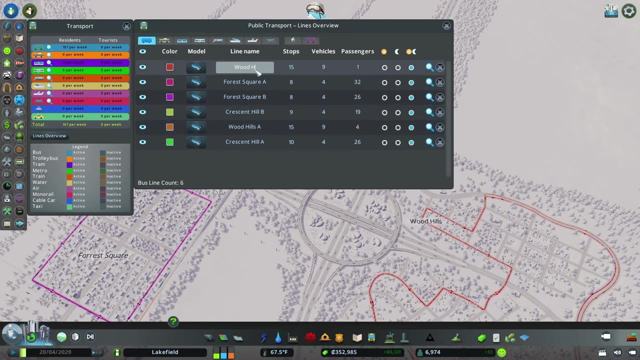 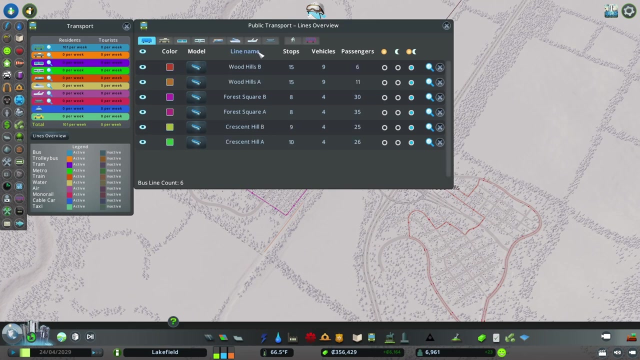 so here, why don't we do? maybe a shade of orange and maybe a darker shade of orange, almost like a red. all right, so let's take a look at our lines overview. so now I did click on lines name and it gives me an in alphabetical order. 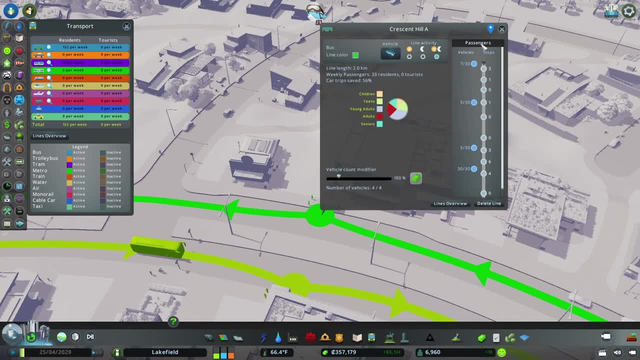 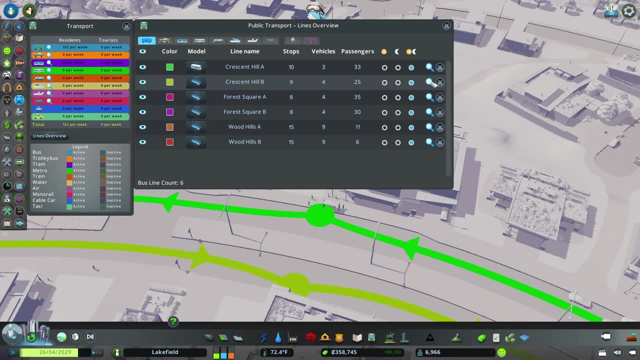 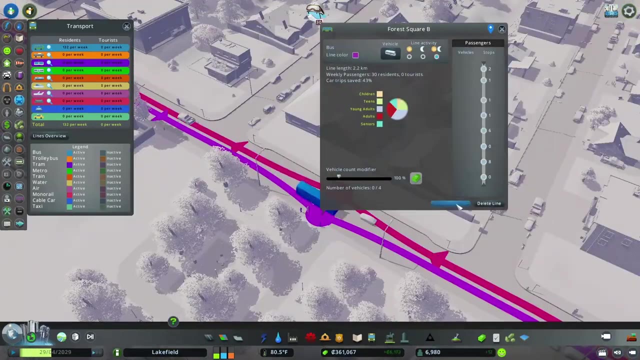 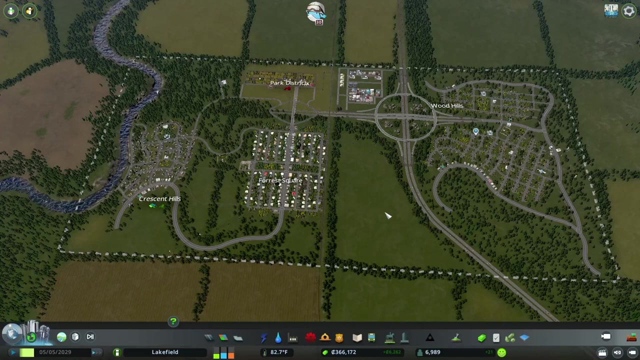 I'm just going to go here and I'm just going to see what kind of buses we're using. so I'm thinking mini buses would be a great option for all of these areas because they're not very big. all right, so now that we got the main routes done in each of the neighborhoods, we're going. 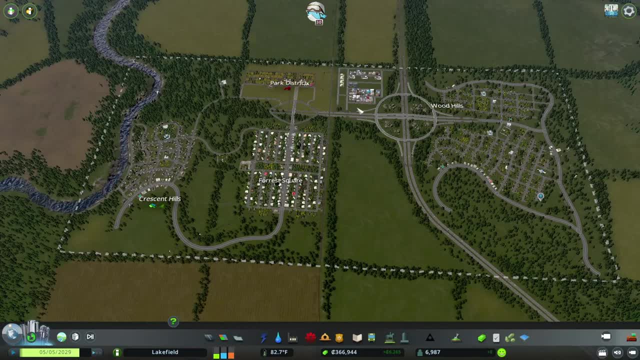 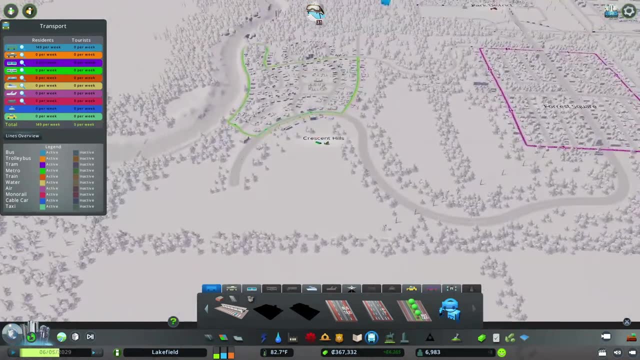 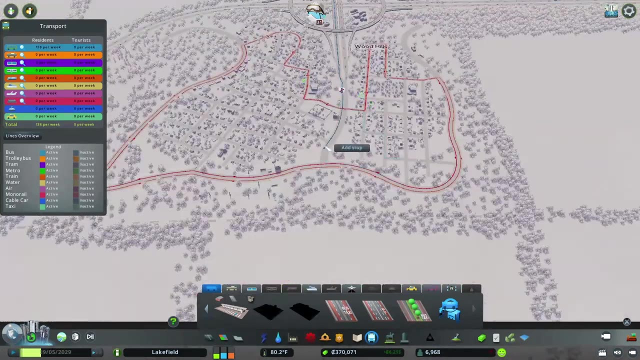 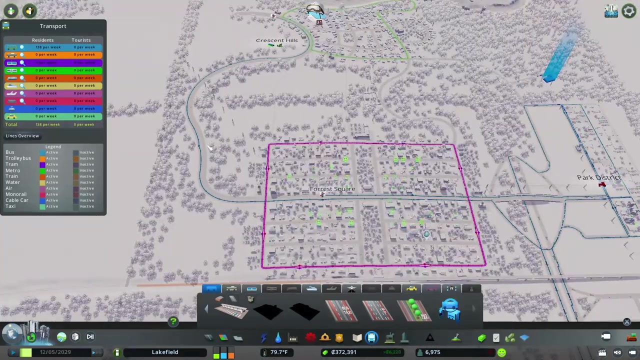 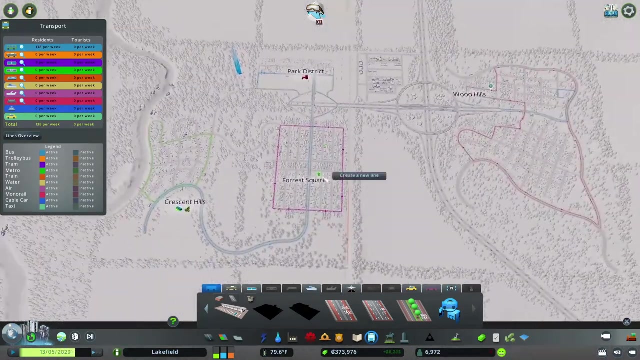 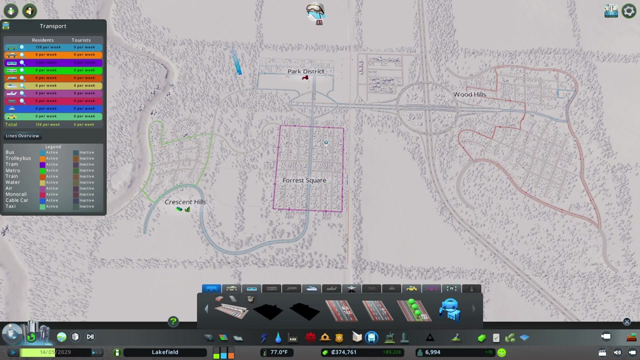 to have a bus that comes through and brings our citizens from one place to another. so let's go back into transportation routes and run a route, all right. so we're going to leave this bus line blue and it's going to be able to bring our citizens all throughout the whole city here, and we're going to go. 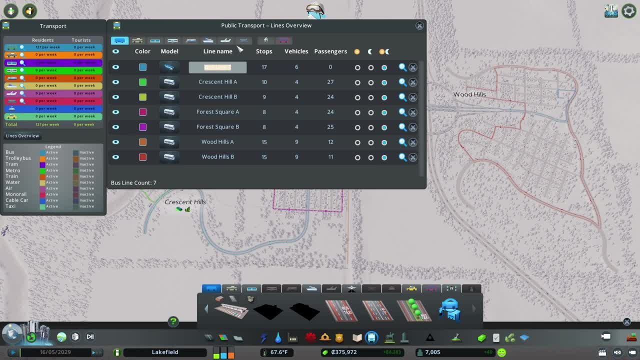 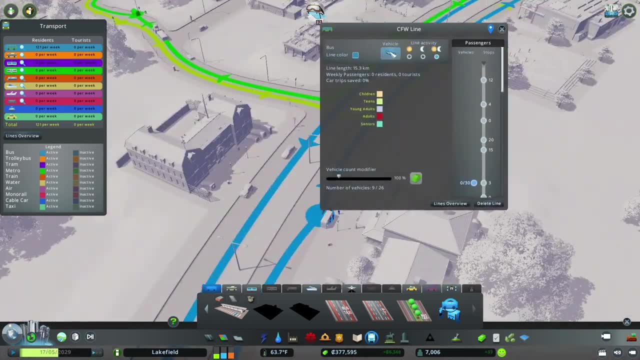 ahead and name this route cfw line. we're also going to go ahead and inspect this line and I think what we'll do is we'll use super bendy buses. this could get quite full, bringing people back and forth, and we'll keep an eye on it, so this should be our busiest bus. so we're going to go ahead and name this route CFW Line. 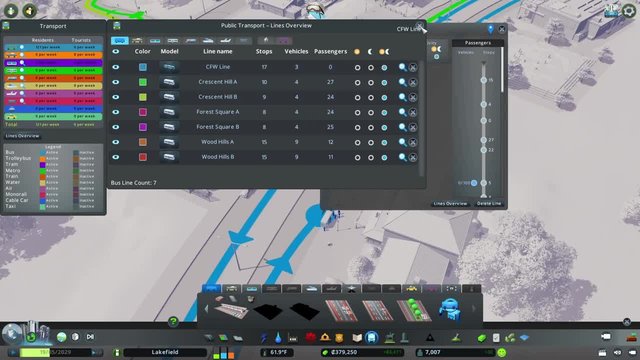 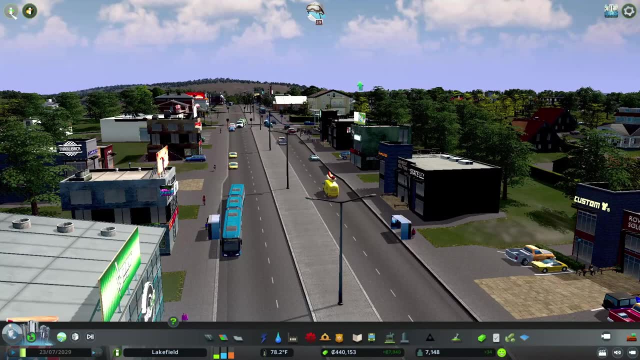 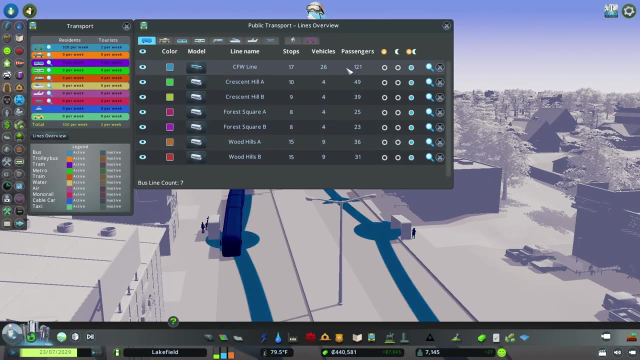 line. we'll see how it goes. so we're gonna let this run for a little bit and I'll be right back. all right, so I let this run for a little bit. we're gonna go in and check on our lines and see how they're doing so. as expected, the CFW. 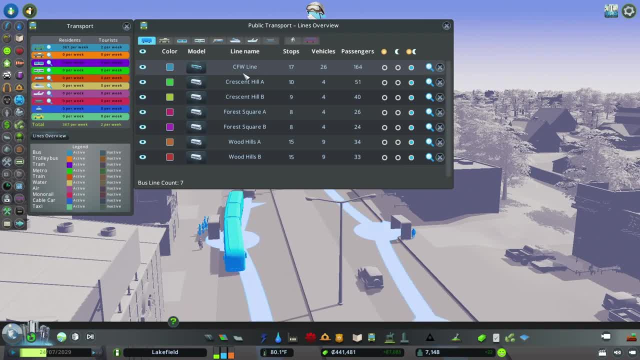 line that's bringing everybody back and forth between the neighborhoods is really cranked up. they're doing a lot of business and that's fine. eventually we may want to put in Metro or something like that, but for this episode we're doing buses. so, yeah, I'm gonna leave this episode off here. I hope you enjoyed and. 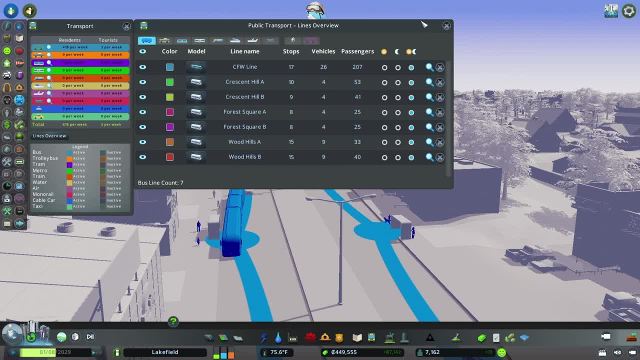 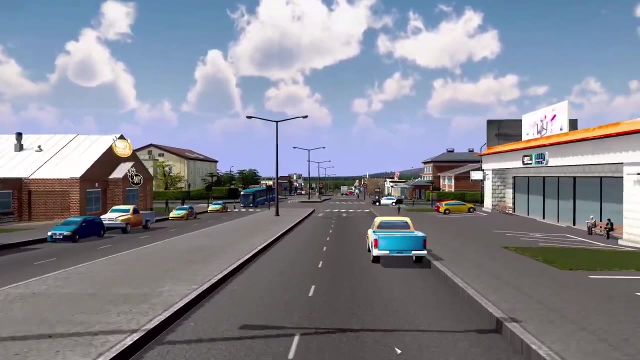 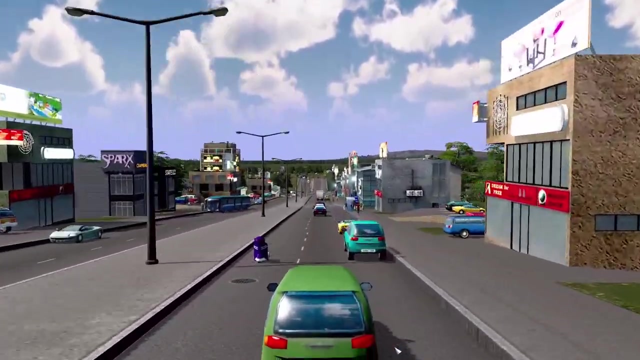 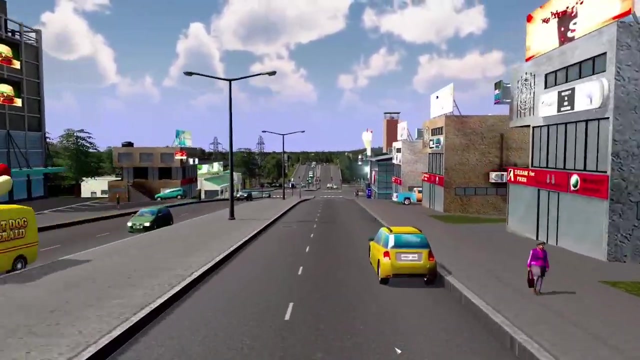 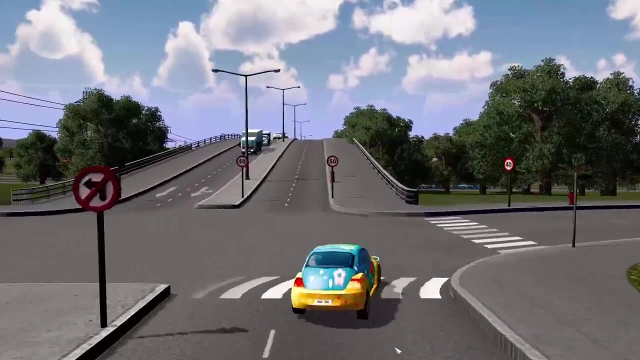 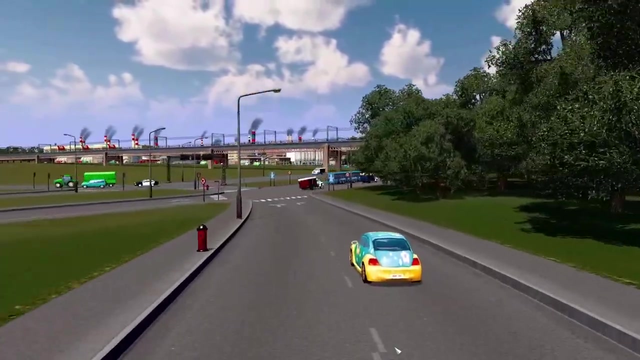 I think we'll take a little bus ride around town and, as always, if you like my content, you want to see more. please click the like button. subscribe, comment, share. do all those good things. I really do appreciate it, and let's get on a bus, so so. 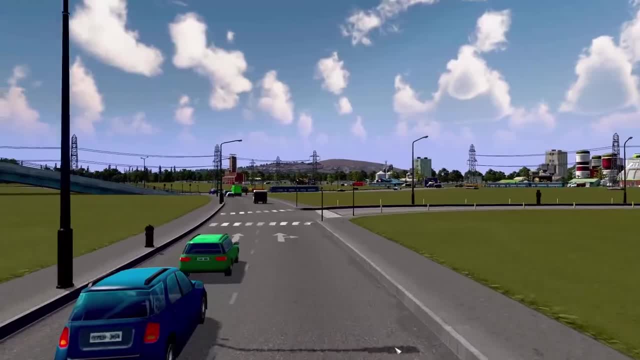 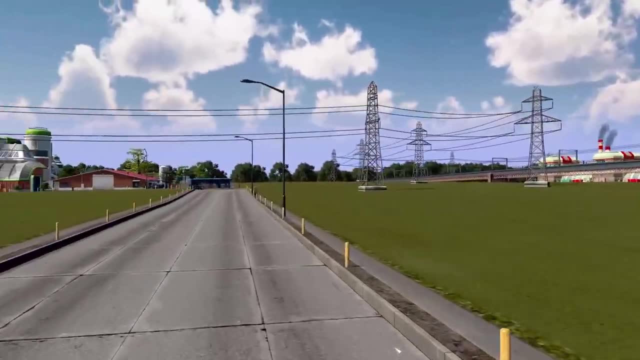 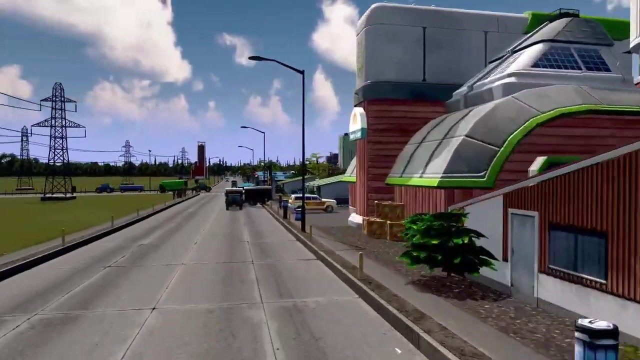 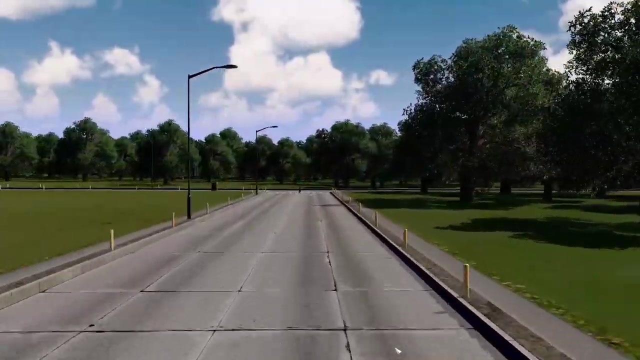 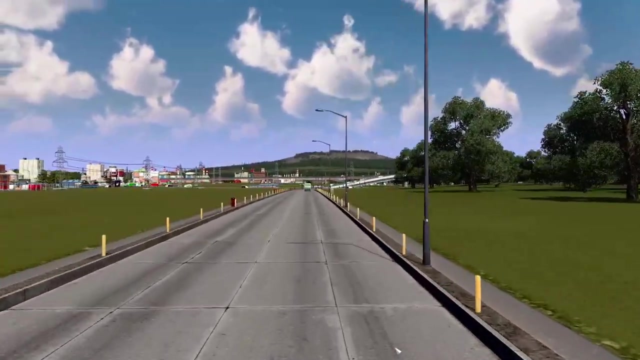 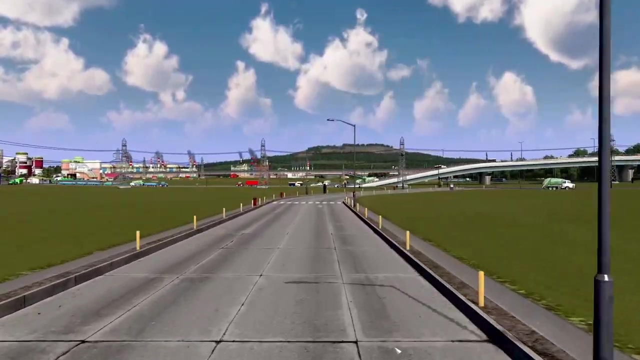 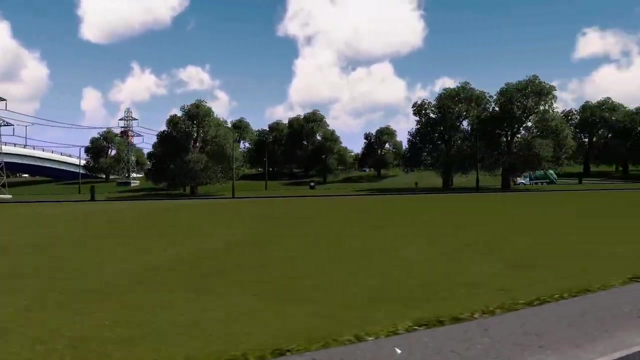